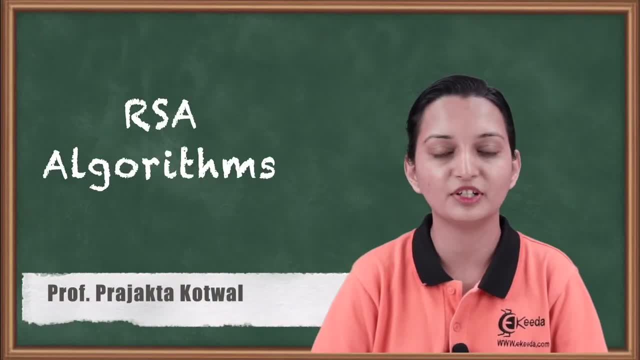 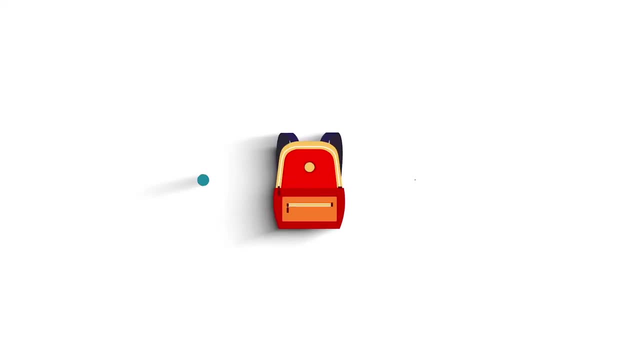 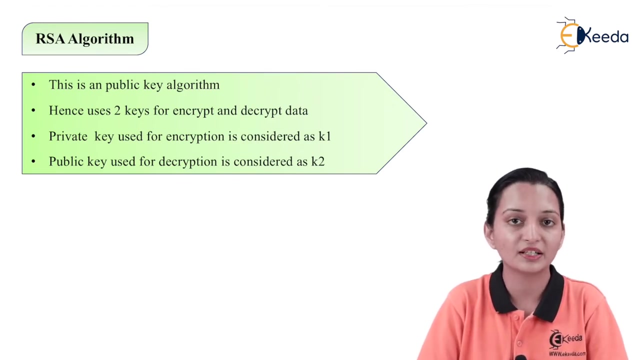 hello friends, in this particular video lecture we will try to understand the theorem which is known as RSA algorithm, along with some example. so basically what it means by RSA algorithm. it will gives us the support to calculate the values for the public key cryptography. so what it means by public key. 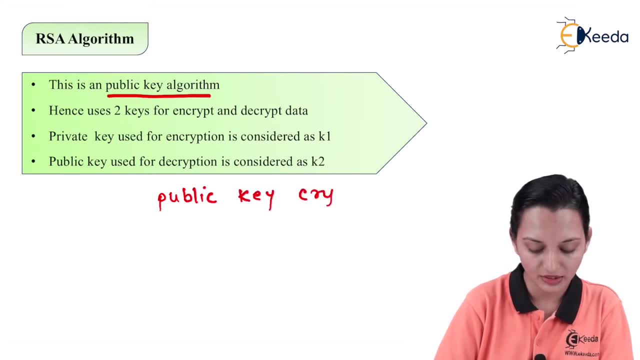 cryptography. we are familiar with the term cryptography. cryptography is nothing but conversion of a one form to the other form, and so that our message will become secret message. so converting the input into some form of the output is known as encryption, and again converting the other form of that. 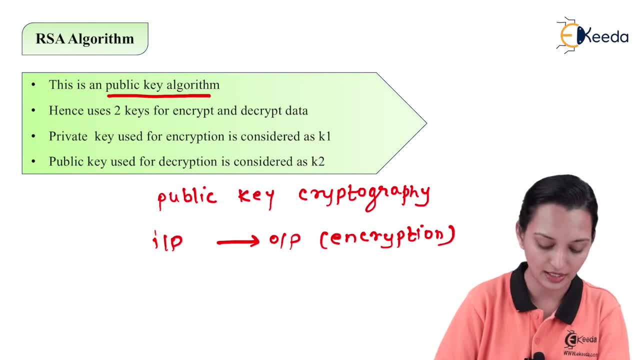 particular output into the original message. that means, if I want to decrypt the message, that means if I want to catch the original message as it is, then conversion from output to input is nothing but decryption. so the process of encryption and decryption- encryption combinedly- known as cryptography. So this is nothing but the term cryptography. 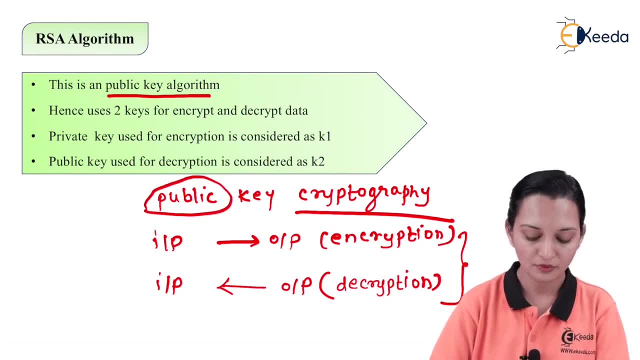 Now what it means by the public key cryptography. Whenever, for the process of encryption and decryption, we are going to use the different keys, then that particular algorithm is known as the public key cryptography. So here for the process of the encryption, the sender or receiver. 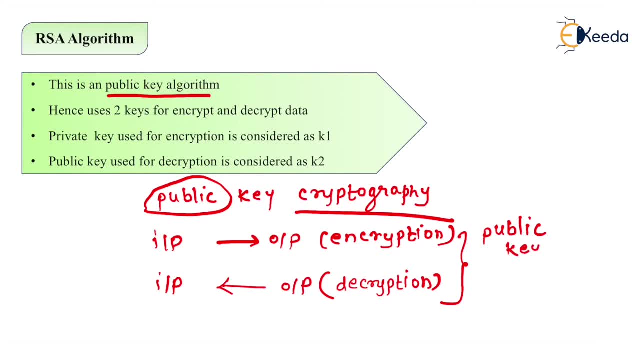 both can use the public key, but for the process of decryption only receiver is able to use a key which is known as private key, And hence here both the keys are used, but they are not going to exchange the private key, so that this particular message transmission is much more secure than that. 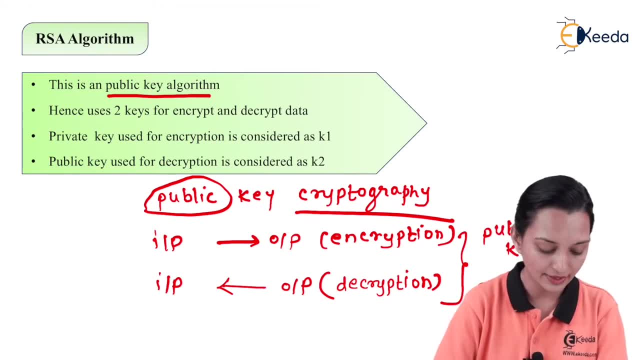 of the private key cryptography, And so it is very essential to study the RSA algorithm, which is going to support the public key algorithm. that means public key cryptography. Hence, as it will use public key, it uses the two keys for encryption and decryption. Private key is 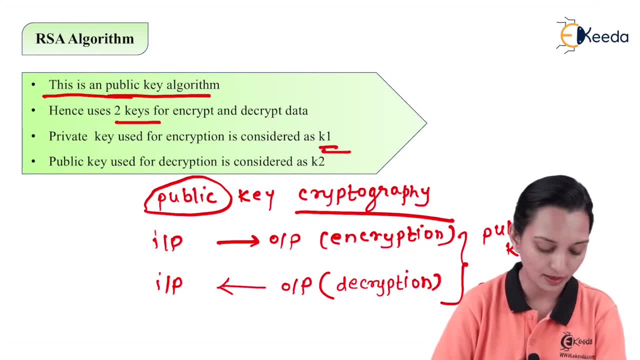 used for the encryption: consider as K1,. public key is used for the decryption: consider as K2.. So the public key and private key, both are going to used, and private key is known as K1 and public key is used as K2.. 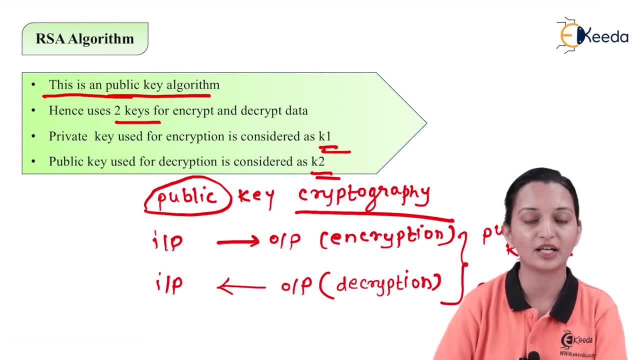 known as k2.. Hence, here we are interested to calculate the values of k1 as well as k2, to find out the input and output. Now we all know that in the cryptographic language the input is known as plain text and the output is known as ciphertext. So to convert plain text into ciphertext, we are 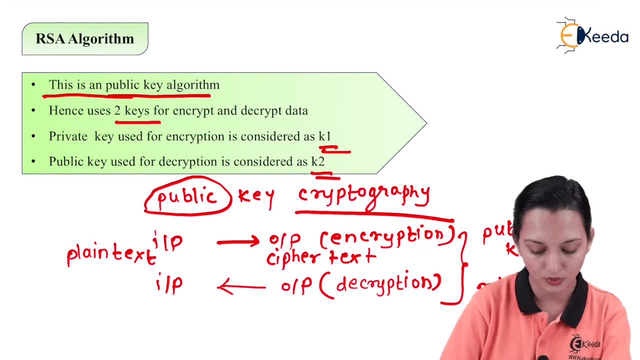 going to use public key, that is k2, and to convert ciphertext into the plain text, we are going to use the private key, that is k1.. So, with the help of k1 and k2, now our aim is to calculate the plain text and ciphertext. So if keys are in your hand, how can you get back your message into the original? 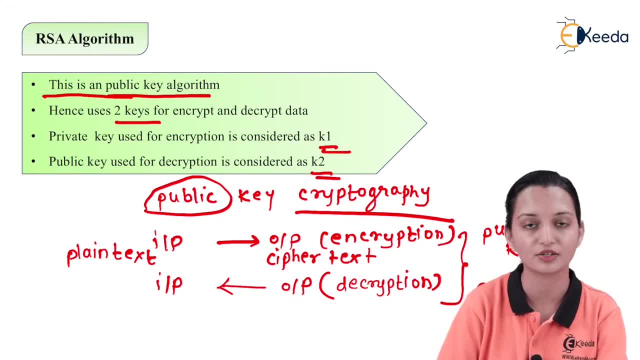 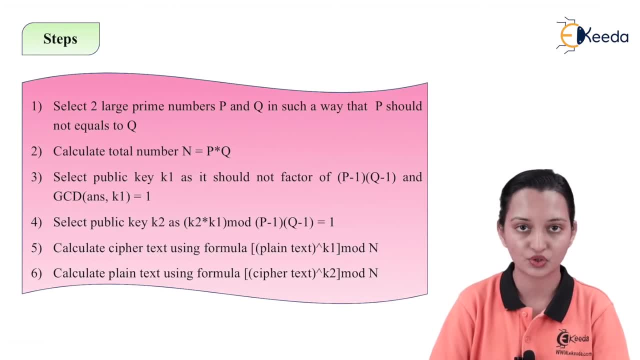 form. How can you encrypt the message? How can you decrypt the message? This is nothing but a total basic idea behind RSA algorithm. So there are few steps to calculate the RSA algorithm. What are they? First of all, select the large prime numbers p and q in such a way that p should not equals to q. So this is the 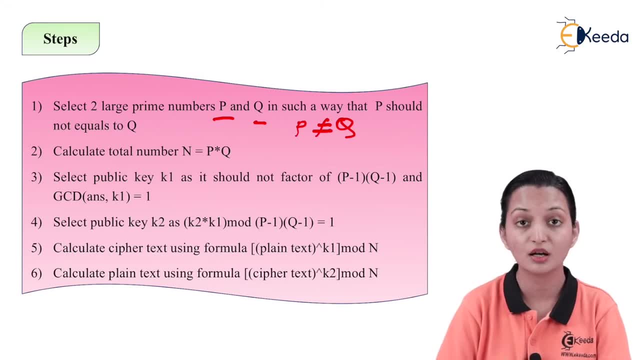 first condition that we required to select the two numbers: both should be prime. So this is again one condition. and prime means what? Who? GCD is 1. So, and both are not equals to each other, So both the numbers should be different. Then step number two: calculate the total number. n is 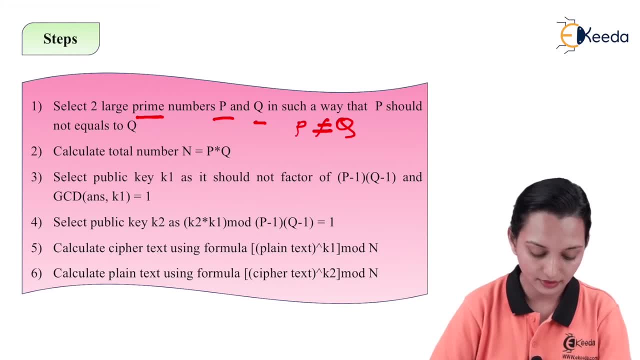 equal to p into q. Three select public key: k1 as it should not the factor of p minus 1 into q minus 1 and GCD of this answer. p minus 1 into q minus 1 will be the answer and GCD of answer and public. 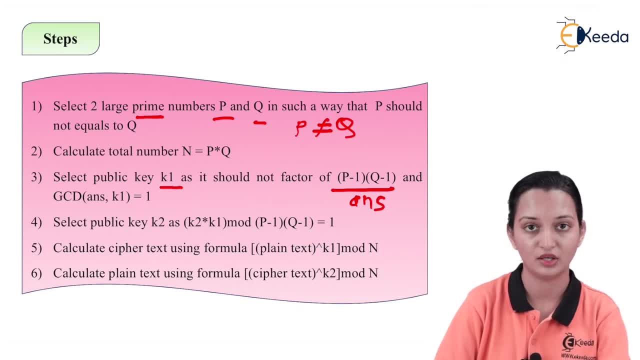 key, that is k1.. So this is the step number three, that once you will calculate n- that is nothing but p into q- you have to again go and calculate p minus 1 into q minus 1, and that answers and GCD of k1. 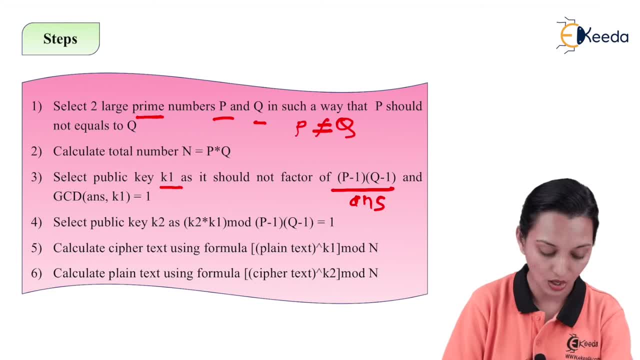 should be 1.. So this is the third step. Fourth one is select public key k2 in such a way that k2 into k1, mod of p minus 1, into q minus 1.. So this is the third step. So this is the third step. 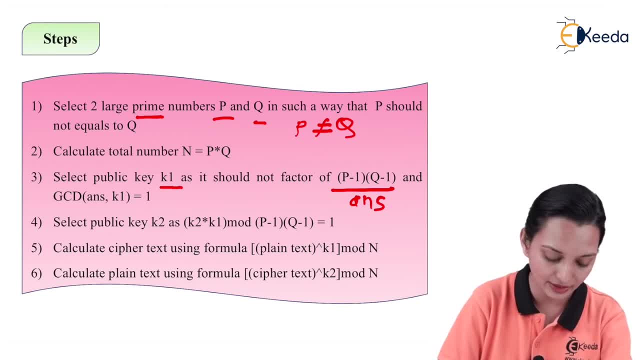 Fourth one is select public key. k2 into q minus 1. into q minus 1 should be 1.. Now we are having k1 in our hand. k1 we have calculate in the step number three. So we are having k1 in our hand. So now we 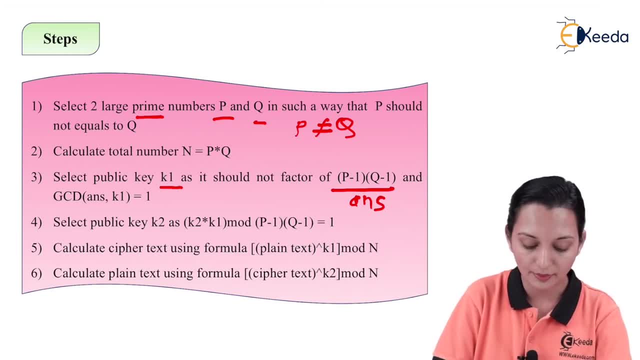 are interested to find out: k2 into k1. mod p minus 1 into q minus 1 should be equals to 1.. We are having p in our hand, q we know, k1 we know. So, with the help of this particular equation, we are able. 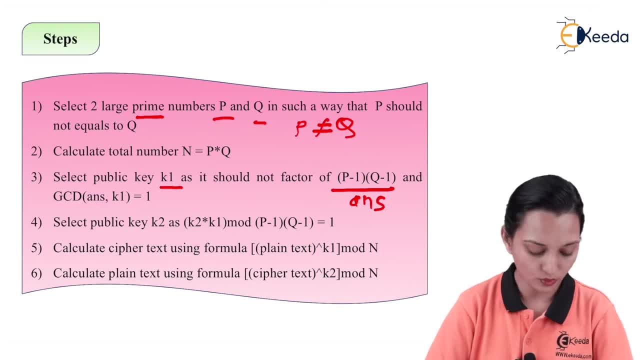 to find out the answer for k2.. Step number four: select public key k2 into q minus 1, into q minus 1.. k2 adds k2 into k1 mod of p minus 1. q minus 1 is equal to 1.. So we are having p, q and k1 in our 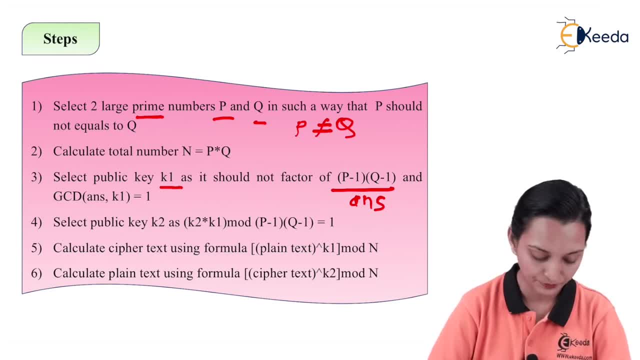 hand and we are interested to find out the value of k2.. Next one: calculate the ciphertext using the formula plaintext raised to k1 mod n. Now we are having k2 in our hand, So we are able to calculate the ciphertext and plaintext. So, using the plaintext which is given in your example, we are 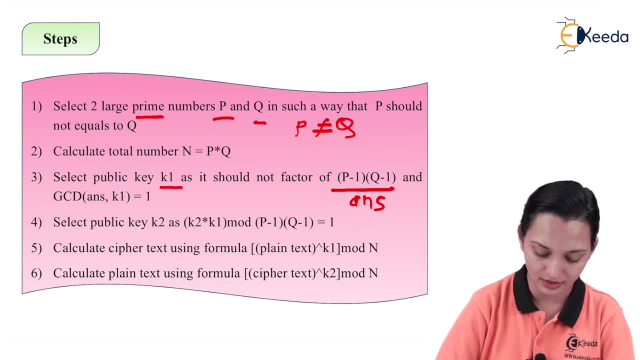 to calculate what ciphertext and using the ciphertext value again, we are able to verify whether our answers are correct or not. Why? Because using the ciphertext, we are again able to calculate the plaintext and which is given in our example. So let us try to understand all the 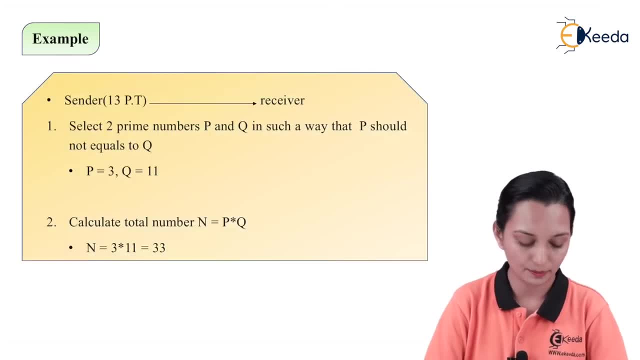 steps with the help of a simple example. So the example is sender and receiver. Sender try to transmit some message with the help of the plaintext. So this is the plaintext. How many bits? or what is the value of the plaintext? 13 is the value of the plaintext Now. 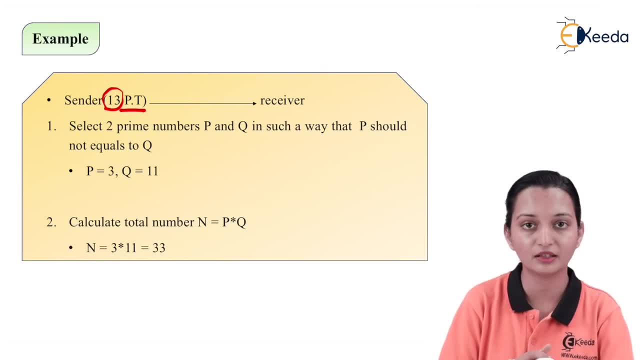 13 is. the value means how many bits are present in the plaintext. 13 bits are present in the plaintext, So the size of the plaintext. that idea is given to us. Now select two prime numbers, p and q, in such a way that p should not equals to q. That was our step number one. So what we have to 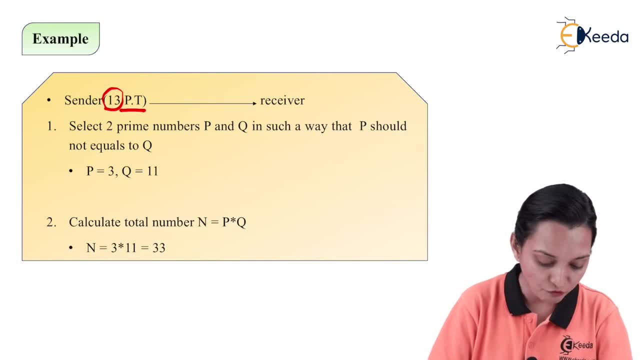 do? What is our aim? Our final aim is to find out the value of the plaintext. So let us try to calculate the ciphertext. So we are having the value of plaintext. Now we are interested to calculate the value of the ciphertext. That means how many bits will be present in the ciphertext. 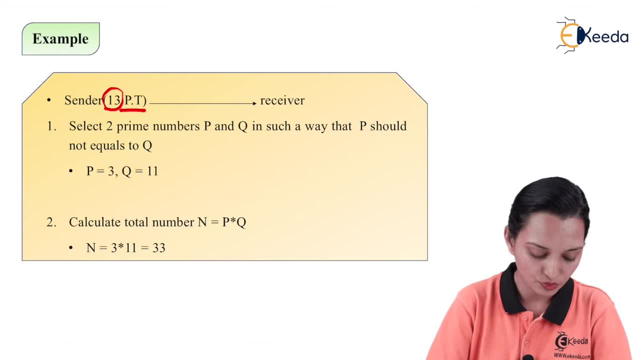 So I will try to select the two prime numbers, p and q. So let us consider: p is equal to 3 and q is equal to 11.. Why? Because 3 and 11 both are prime and both are not equals to each other. So 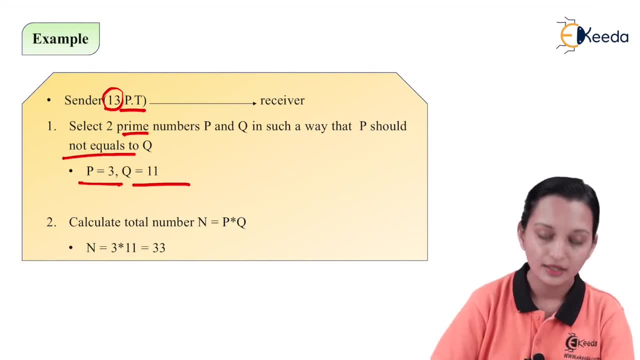 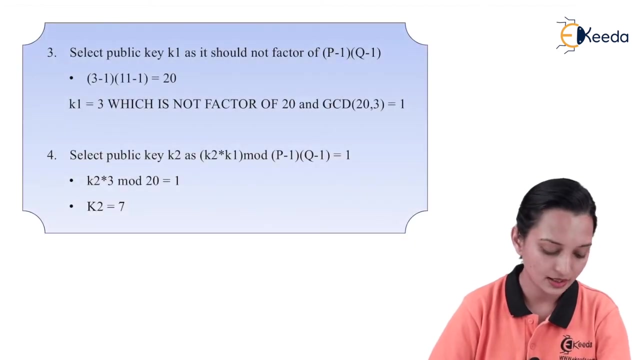 both the conditions are get satisfied. Second, calculate number n in such a way that n is equal to p into q. So here n is equal to p is 3 and q is 11.. So 3 into 11 is equal to 33.. So this is our step number. second Step number three is select public key k1. 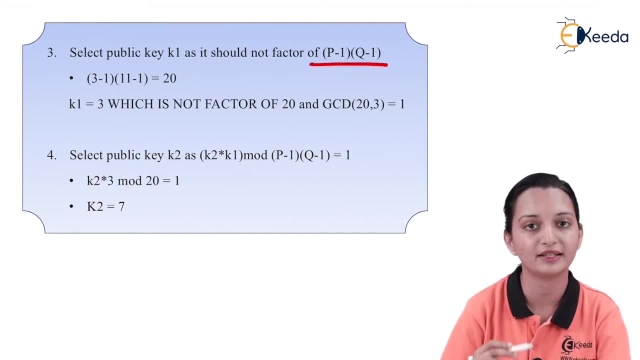 as it should, not the factor of p minus 1 into q minus 1.. So what? I have to select a public key. So first of all I will try to calculate p minus 1 into q minus 1.. So we all know that value of p is. 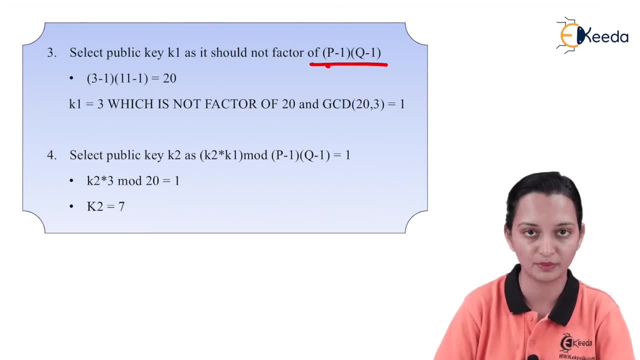 3 and q is 11, which we have considered in the step number one. So 3 minus 1 into 11 minus 1, that is, 2 into 10, is equal to 20.. So we are getting such kind of answer. Now we are interested to find. 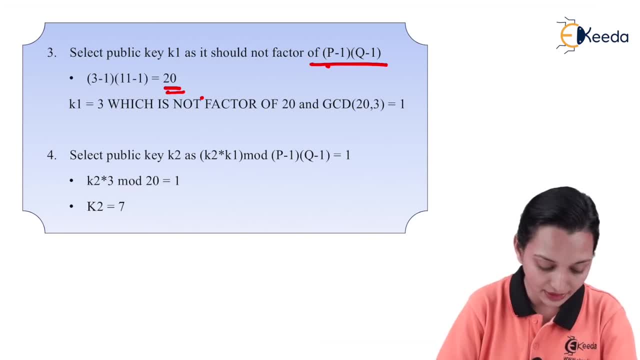 out the value of k1.. How can we calculate? We have to find out such a value which is not a factor of 20, and the gcd of that value, and 3 should be 1.. Why 3? Because that particular key I am going to. 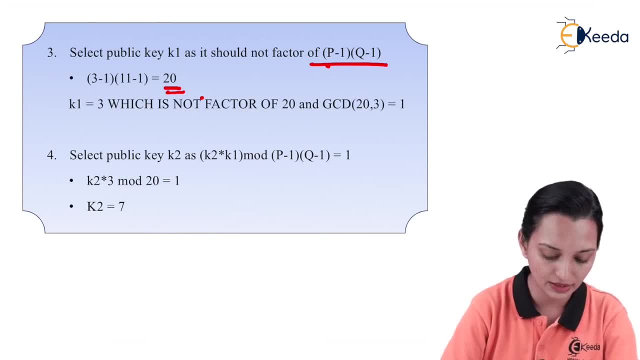 select as 3.. Why? I will tell you The factors of 20 if I want to calculate the factors of 20.. How can I calculate it? 20 into 1.. Second is 10 into 2.. Third is 4 into 5.. So I cannot calculate more. 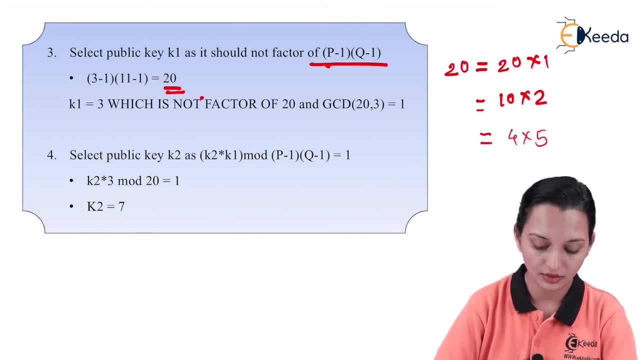 factors rather than this 3.. So here I am going to calculate the factors of 20.. So I am going to. the number 3 is not present in all the factors. So first of all I can select. the value of k1 is equal to 3.. What is the next step? The gcd of answer comma k1.. What is the answer? p minus 1. 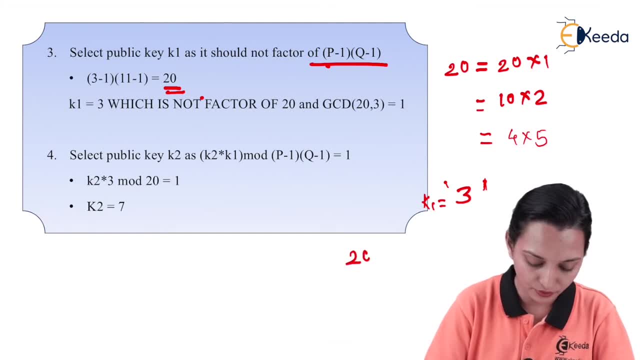 q minus 1 is equal to 20.. So gcd of 20 comma, k1, which we try to select, that must be 1.. If not, then we have to go and select the other key for the k1.. So if you are going to observe the 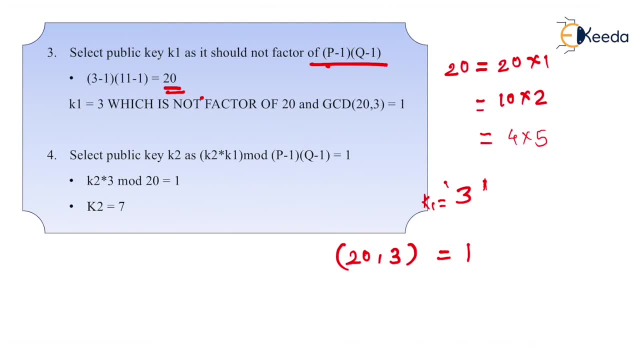 highest greatest common divisor in between 20 and 3 is 1.. So this condition is also get satisfied. So, as the both conditions are get satisfied, First is it is not a cofactor of 20 and gcd of 20 comma 3 is 1.. Hence we are able to select. the value of k1 is equal to 3.. Now we are 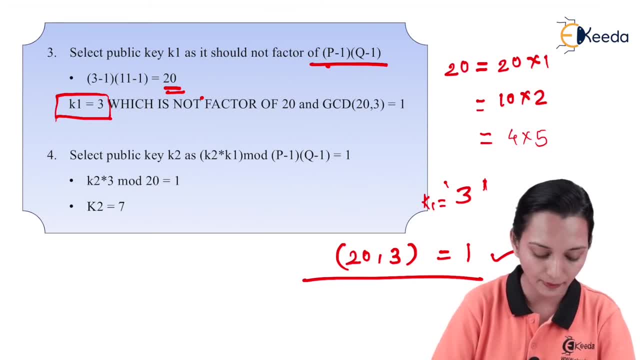 getting the value of k1.. What is the next step? Select public key. This is nothing but what Private key. Now we are interested to select the public key in such a way that k2 into k1 mod of p1 minus q1. 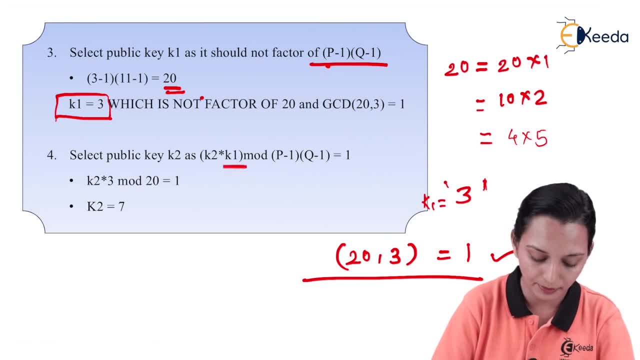 is equal to 1.. So we are having k1, p, q in our hand. We are interested to find out the value of k2.. So k2 into 3 mod of 20 is equal to 1.. Now how can we find out this particular value of k2?? 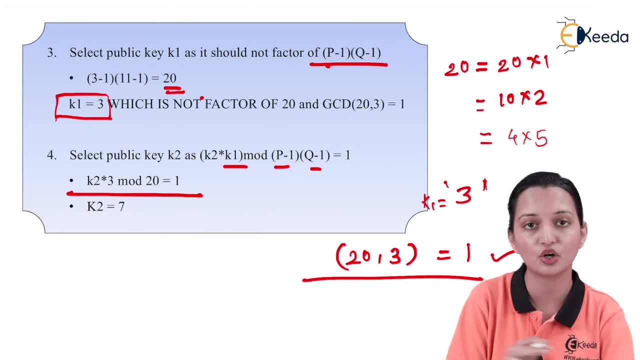 Now try to select the different values of k2 should not be 0. Any key should not be 0, because key is nothing but that particular bits which will provide us to decrypt the message. So k2 can be. first of all, we will try to select. k2 value is equal to 1.. So what will happen if? 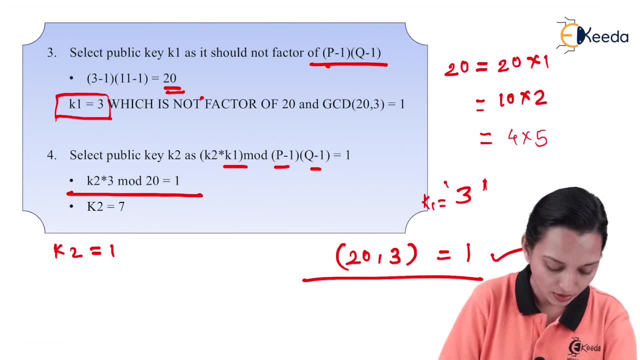 you are going to select, the value of k2 is equal to 1? It implies, try to put up the value 1 into 3, mod of 20 is equal to 1.. Whether it is true If I am going to divide the answer 3 by 20,. 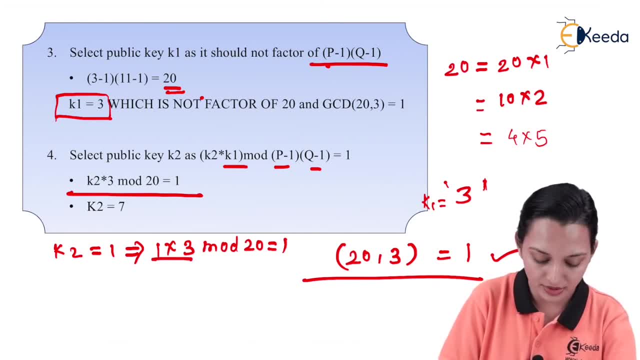 then I will never get the remainder 1. Why? Because this value is less than that of this value. So what we have to do, Try to select the value of k2 in such a way that that answer will give you the greater value than that of 20.. So what can I do? if I am going to select, k2 is equal. 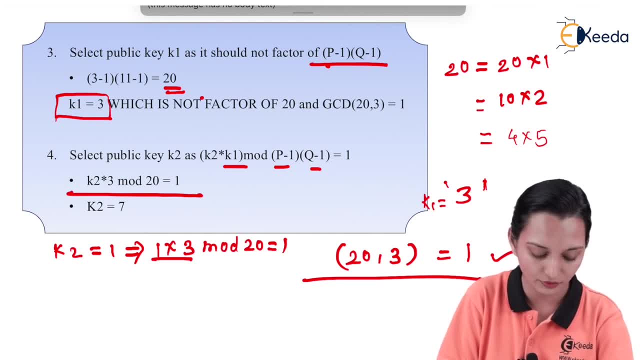 to 2?? I am getting 2 into 3, 6, which is less than 20.. So I will never use that 2.. k2 is equal to 3, 3 into 3, 9- again less than 20.. 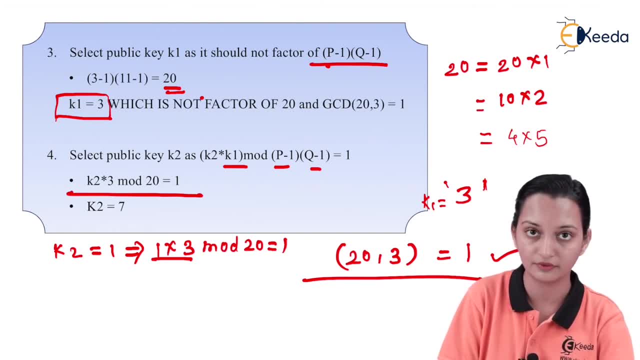 k2. select as a 4, 4 into 3. again, 12 less than 20.. Select k2 is equal to 5, 5 into 3, 15 less than 20.. k2 is equal to 6, 6 into 3,, 18 less than 20.. If you are going to select, k2 is equal to 7,. 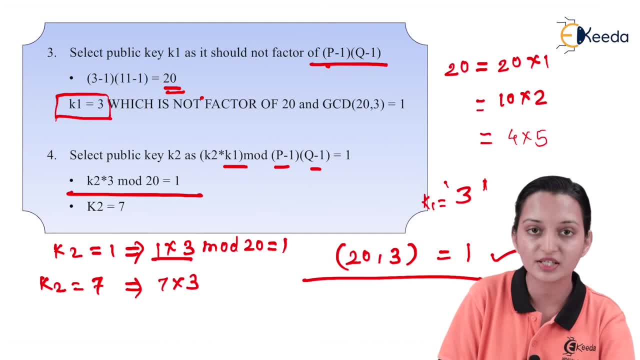 that implies 7 into 3, which is nothing but 21 and which is greater than 20, so that you can divide it. So mod 20 and try to find out whether it is able to satisfy the condition is equal to 1 or not. If not, then you have to go. 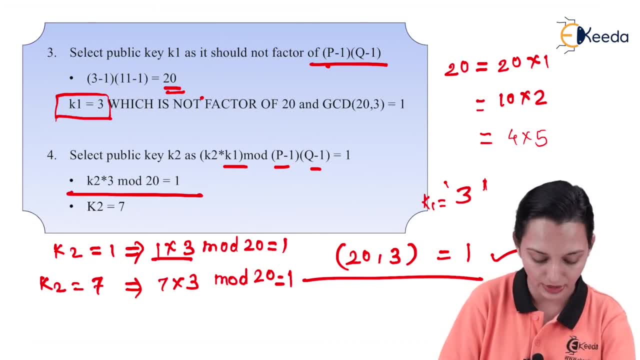 to calculate other value for k2.. But here, if you are going to divide 21 by 20, then we all know that the remainder will be 1. And only and because of this thing the k2 value we can select as 7.. 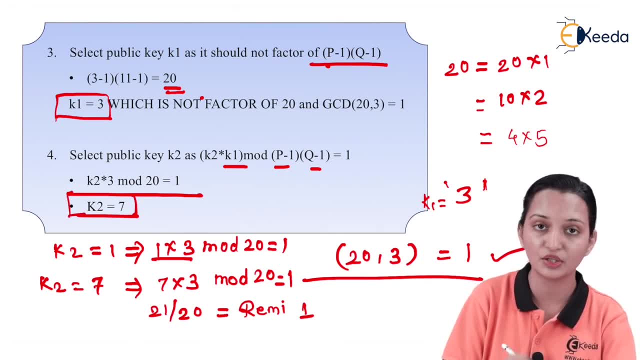 If here you are not getting, remainder is equal to 1, then you have to follow the same procedure again and again up to you are not getting the value 1 of this particular equation. So here the value of k2 is equal to 7, which is nothing but the true condition which is satisfied. 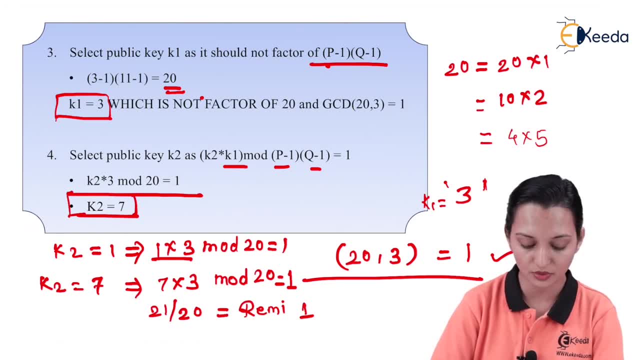 to us. So we have to compute the values up to we are not getting. the remainder is equal to 1.. Why? Because that is nothing but the condition. So value of k1 is become 3,, value of k2 is become 7.. So we have to compute the values up to we are not getting. the remainder is equal to 1.. 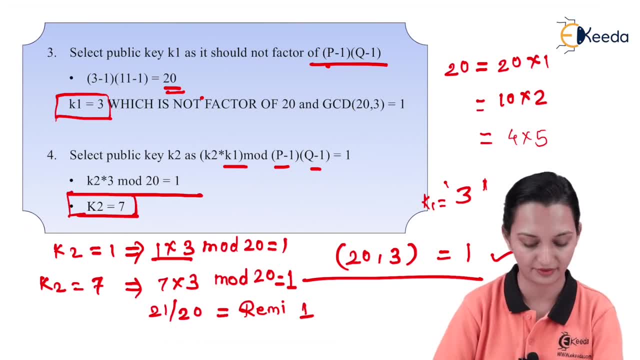 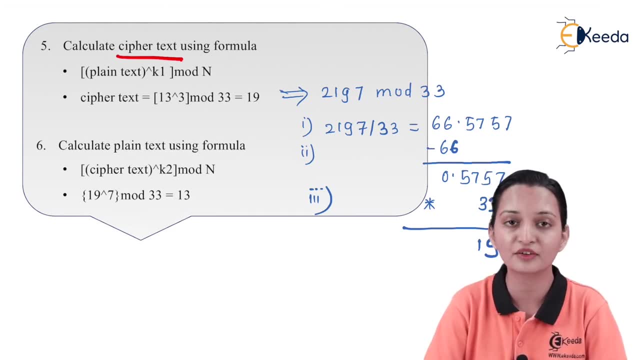 7. So we are getting both the public key as well as private key. So with the help of all that values we are interested to calculate the ciphertext that is actually the encrypted text. Ciphertext can be calculated as plain text raised to k1 mod n, So ciphertext is equal to: 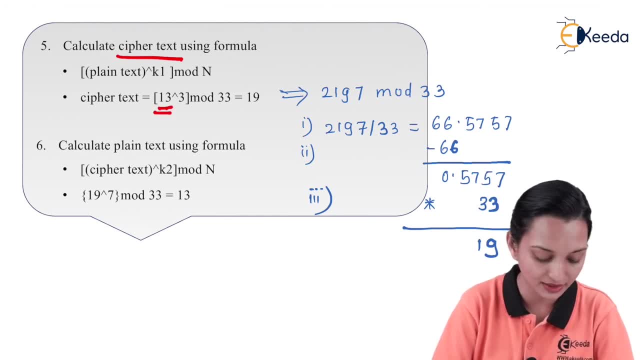 plain text is already given in our example, that is, 13 raised to 3 mod 33.. Now its answer is 19.. How can we calculate this particular value, or the expressions? 13 raised to 3 become 2197.. 2197 mod 33 is our actual calculation. So what we have to do? Divide 2197 by 33.. 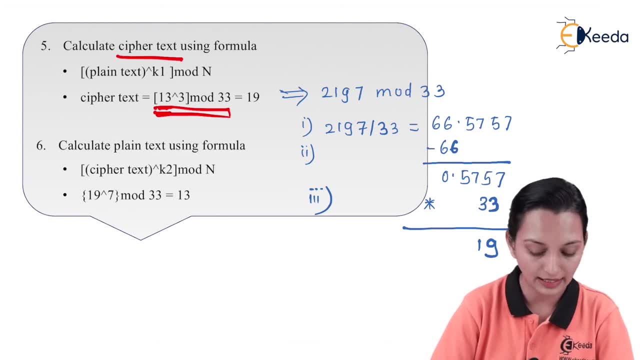 So if you are going to divide it, you will get something That will be 66.5757.. Now subtract the real term of the answer. So what is the real term? 66. So subtract that particular value, Then you will get the answer: 0.5757.. Then multiply with the help. 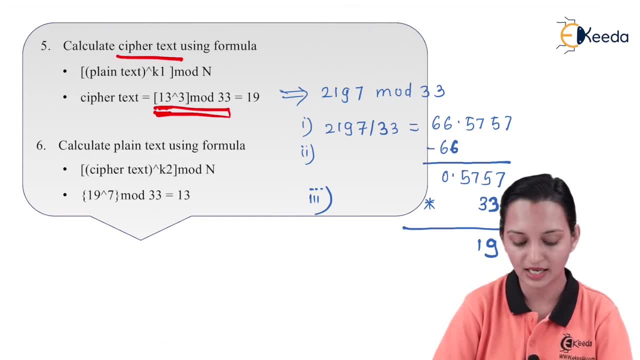 of mod value to that answer. So whose mod we are interested to calculate? 2197 by 33.. So multiply the value 0.5757 by 33. And you will get the final answer That is nothing but 19.. So the ciphertext value is: 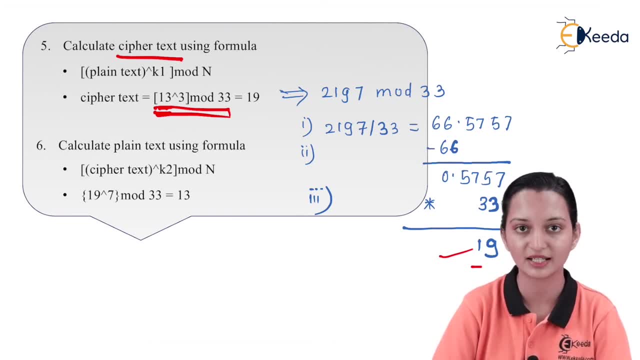 19.. That is, the number of bits present in the ciphertext are 19.. Now you are here getting the actual answer, But if I want to verify whether I am getting the answer is correct or not, then I can verify it by calculating plain text. Why? Because plain text value is already given. 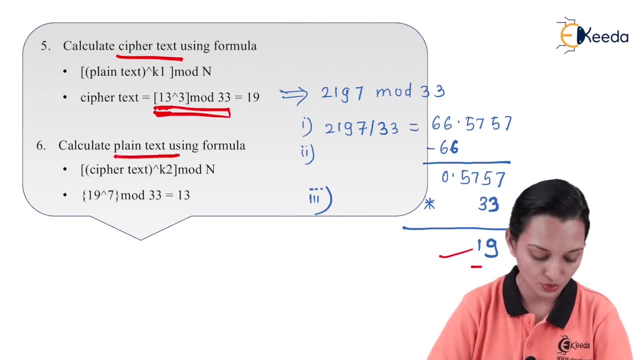 in the example And that is what. That is: 0.5757.. So if I want to verify that, then I can verify that. So if I am going to verify the answer, how can I verify? Plain text can be calculated as: 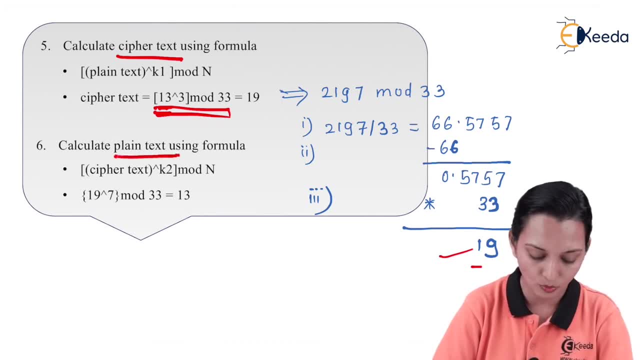 ciphertext raised to k2 mod n, The value of k2 was 7.. What we have calculated, The value of ciphertext, was 19.. Just, we achieved that value. So 19 raised to 7 mod 33.. Again, you have to. 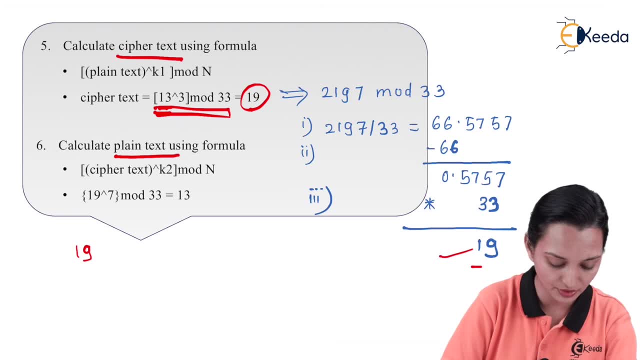 follow this procedure, That is, you have to first of all follow the 19 raised to 7. That, then that answer you required to divide by 33.. You will get again some answer. So in that, subtract the real terms and you are getting point answer. That means 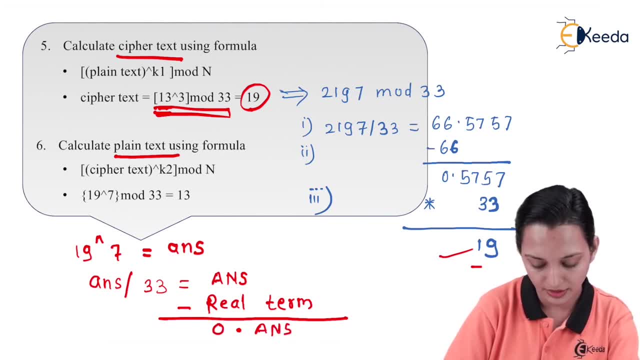 0 point, some answer. So finally, multiply this answer by 33.. You will get the answer 13.. so, same procedure, or the steps which we have used for the calculation of this 2197 mod 33, that same steps we have to use for the calculation of 19 rest to 7 mod 33 and you are getting the 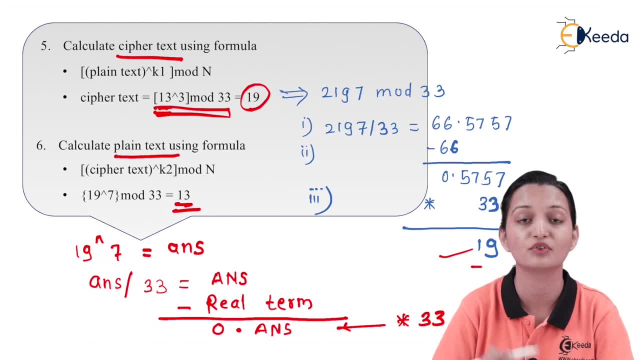 answer 13 and which is nothing but what your plain text, which is given in the example. so, with the help of the verification, you are able to say that the answer of a cipher text is correct. why? because after put tapping the value of the cipher text, you are getting the, as it is, plain text. so this: 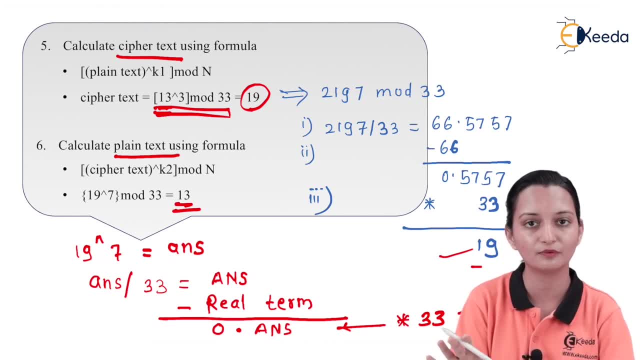 is nothing but what? cryptography? conversion of one form to other form and again get back the previous form as it is with the help of decryption. so both the process of encryption and decryption are getting satisfied over here. so what is the conclusion? with the help of this example, 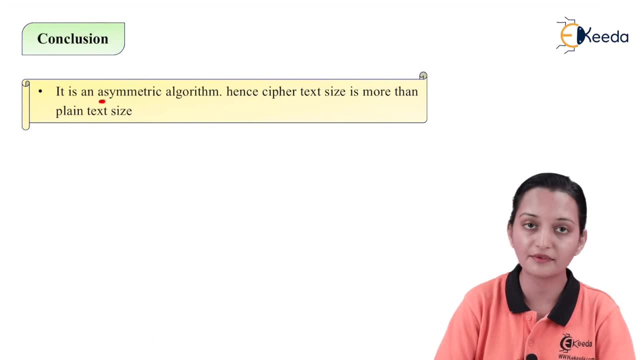 it is an asymmetric algorithm. what we have stated in the first slide. that That is. it is the asymmetric cryptography, that is, the public key cryptography. Why? Because it uses the two keys for the encryption and decryption process, and hence it is also known as the asymmetric algorithm. 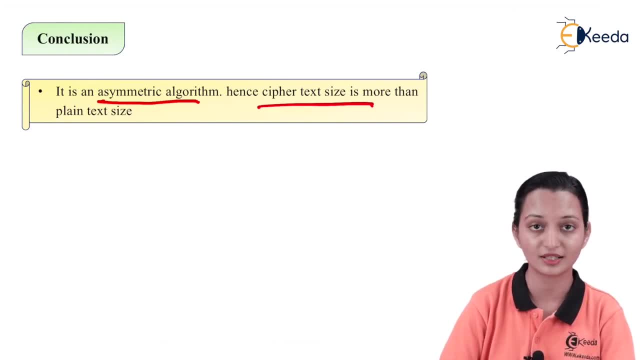 Hence ciphertext size. what is the value or the size of the ciphertext 19,, which is more than that of the plaintext size? The plaintext value is 13.. So the asymmetric algorithm is nothing but the public key, cryptography, and here this: 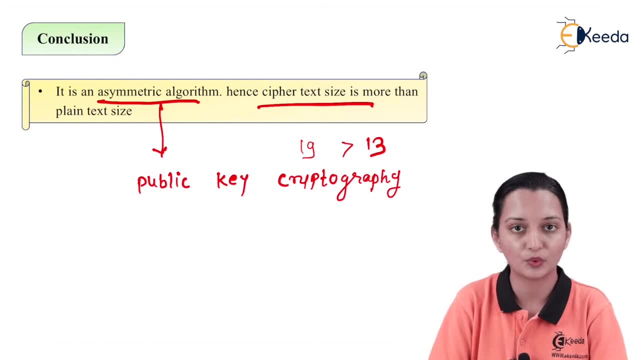 says that if you are going to use the public key cryptography for the encryption and decryption process, then you are achieving the ciphertext size is more than that of the plaintext size. and, yes, you are going to satisfy the condition. Why? Because ciphertext size is 19 in our example and plaintext size is 13, and both the ways.